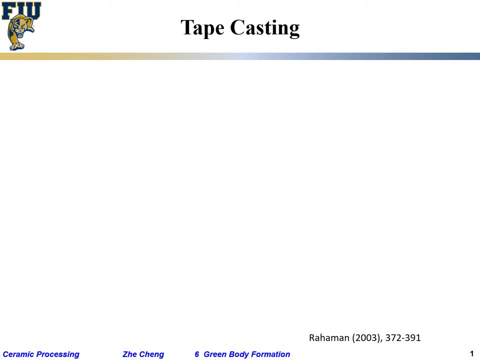 let's just continue a little bit. tape casting, which is related to casting, but cast the slurry onto a so-called carrier, film carrier tape- to to get it and to control the thickness. you just control the, the gap between your so-called blade, just the the thing that. 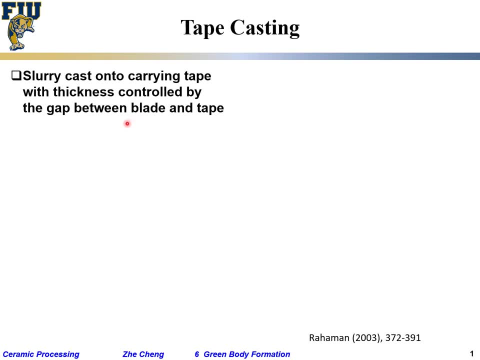 you use for moving scraping versus your carrier tape. okay, here we are showing a schematic. you see, we have this tape that is rotating and then we have slip contained in this container. at the bottom of this container the slip would flow out, and how much will it flow out, depending on my 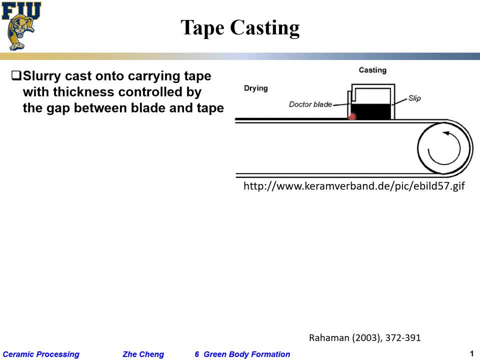 so-called doctor blade position or the gap between the tip of the doctor blade and your carrier film make sense. if i leave it all the way up, all the slurry come out quickly. of course, depending on the viscosity, it may not maintain that thickness, but, as you can imagine, when i go to thinner and thinner, thinner i'm going to, in principle, get. 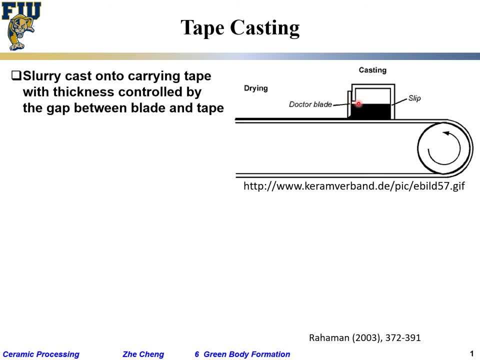 thinner and thinner slurry until to the extent that the surface tension prevented to go away make sense. when that, when the slip, the gap is too small, no thing can flow out because the surface tension is enough to hold it make sense. so that's kind of like. but 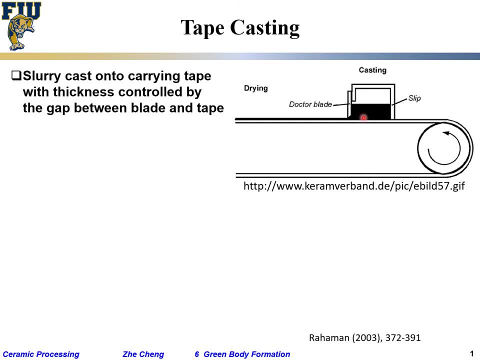 in within extent. you can control it: the thickness, not super precision control, but roughly you can control whether, whether it's 10 micron versus like, let's say, 20, 30 microns. and of course you can do this multiple times: cast and cast another layer. oh, you can cast a thin layer. 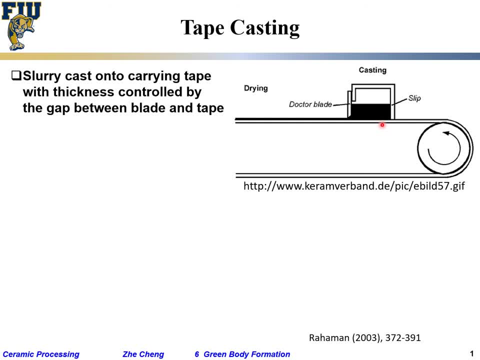 and then machining, laminate thinner layer together to get a thicker layer. do you see what i mean? i can cast a thinner layer and cast another thinner layer and then, machining, laminate, put two layers together, pass thin them through a roller and then i get a thicker layer. okay, so use for the production. 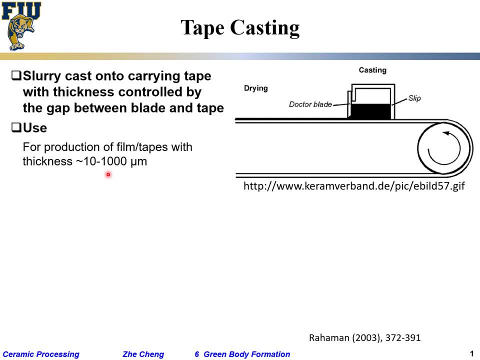 of film or tape with thickness from 10 micron all the way roughly to one millimeter. okay, the slurry formulation. consideration: solvents: you want to use solvent. traditionally people use organic solvent: isotone, mek for thin tapes, phthalene for thicker paste. but these are organic solvent more expensive and smelly and also. 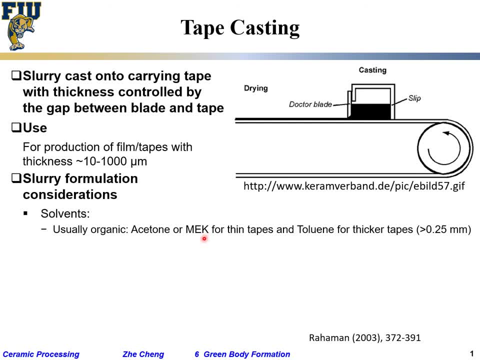 you have fire hazard. make sense fire hazard? all these are combustible, flammable or even explosive organic compounds which you try to do them. if you have to do them, do them with care. it's getting more and more common to use aqueous based solvent. aqueous based system: cheaper, less smell, okay, more friendly. ceramic content: typically 30 to 80 percent. 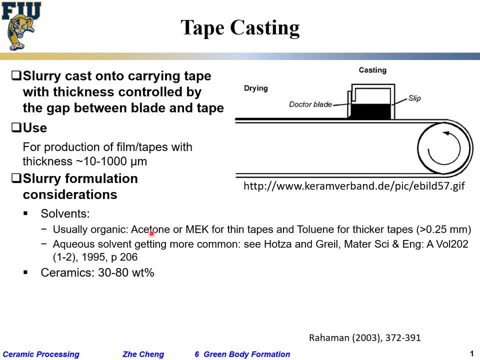 in the slip and اللат, depending on your process condition. you see, that's a big window. that's a big window. what is exactly you use? well, depending on- i guess most likely you're not the first one to do it- depending on your history, depending on your tradition, depending on your 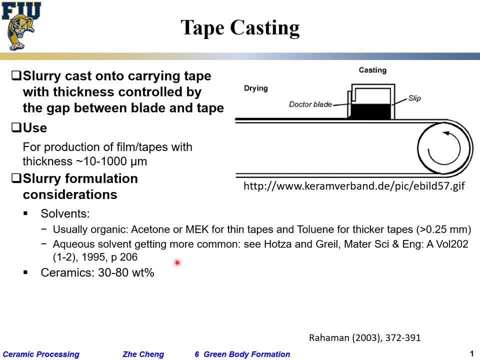 quality whether you do some minor adjustment. okay, binder, the polymer bander you added. that gives it's the plastic property. you can bend it back and forth, because ceramic wind body without binder it's not going to give you that flexibility. okay, plasticizer, the small molecule that you added into the polymer binder to reduce the 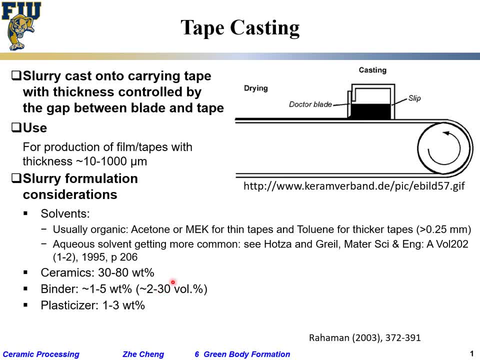 glass transition temperature, essentially to make the polymer more plastic, more flexible, like water or acetylene glycol, something like that. dispersant to help the powders disperse really well dispersant. okay, so these are the numbers and we don't have precise number, precise prescription. 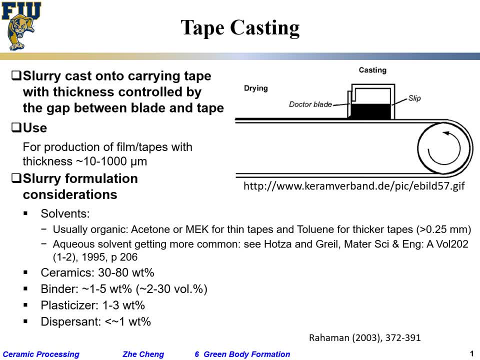 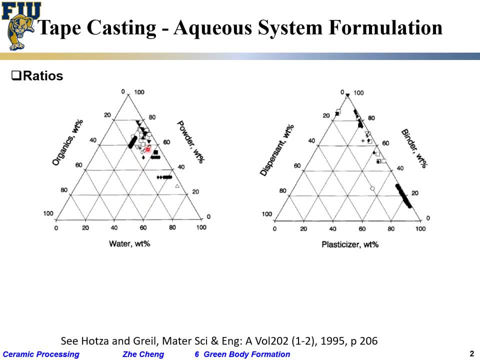 what you are going to do. you try it in the lab also see what literature what other people have been using. okay, so here i'm showing a recipe, kind of like a recipe region, a triangle between organic and non-organic, between powder, between water. that's kind of like your basic, when you do slip casting. 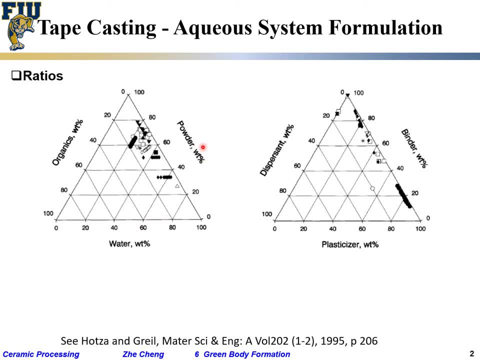 or tape casting, your basic system you have always. essentially, you need ceramic powder, you need solvent and let's say we are using water. let's say we are using water and then all the binder, plus all the binder and the dispersant, we lump them into organics. or even some non-water plasticizer, acetylene glycol, will lump them into organics. 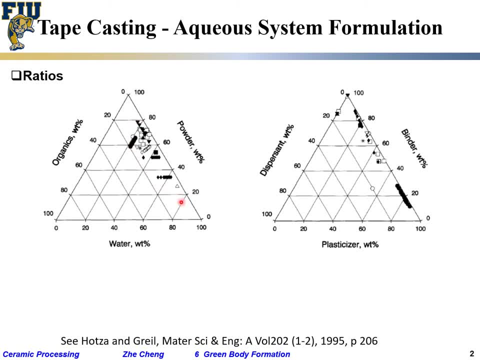 and what we see is: okay, the literature, okay, pulled out a different recipe. and you see, okay, it's quite often in this range, quite often in this range. how do i read this plot? you see, organics, this skill is organics. organics, this skill is organics. 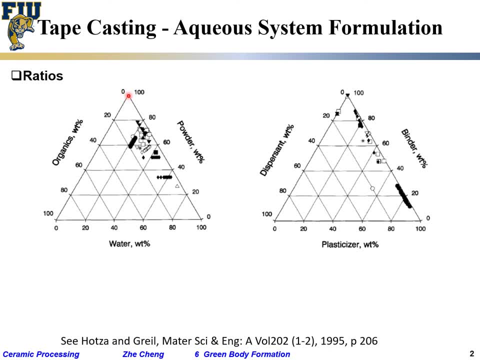 which means, if I'm here, I have what? Zero organics. If I'm following down here, if I'm reaching here, I have 100% organics. If I'm at this point, my system has zero powder, zero water. 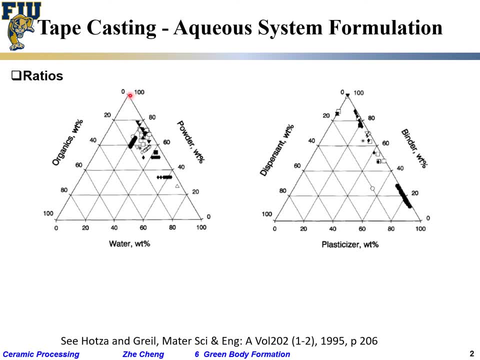 all organics. If I'm at this point, I have what. If I'm at this point, I have what I have: 100% powder, which means have to be zero organics, zero water. 100% powder has to be zero organics, zero water. 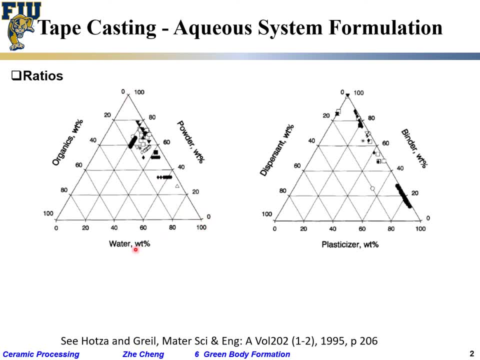 If I'm here, remember this is water scale. If I'm here, I'm 100% water, zero powder, zero organics Make sense. So just keep in mind the three so-called corners. That's very, very important. 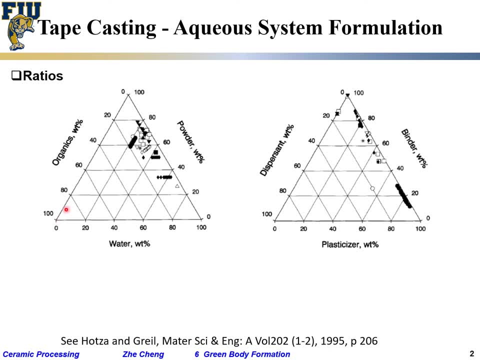 Here I'm all organics, Here I'm all powder, ceramic powder, Here I'm all water. So let's pick something like this point To determine this, to recalibrate this plot like a three-component phase diagram. do you see, if I'm here, I'm roughly 70% of powder by weight. 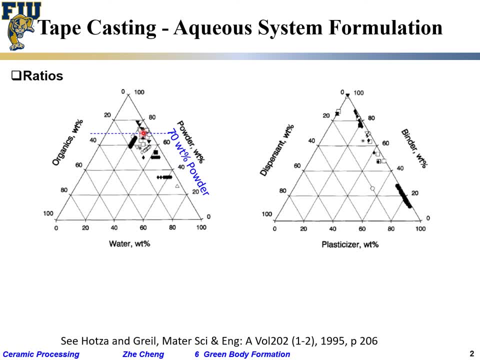 70 weight percent of powder by weight. if I'm pointing this point, Make sense, Because this is 100% of water. Make sense: 80% of powder, I'm here. 80%, 60% in between, I'm 70%. 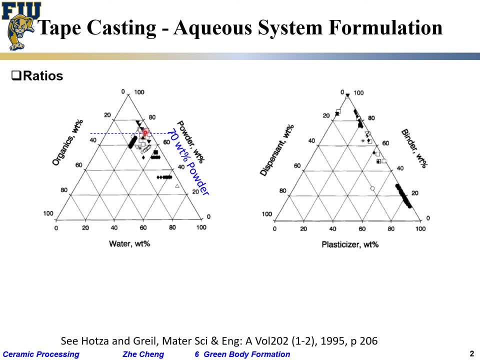 You read the powder on here Make sense. But on the other hand, you may ask Dr Cheng, can I read this for powder? Can I read this scale for powder? No, because this scale is for the left side scale. 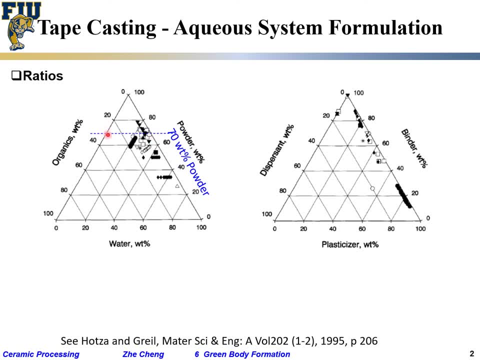 If I'm doing this, okay, I cut here 70,, cut there 30. But if I was thinking of powder, I have to read the powder scale and 70%, 70% of what Powder? But can I read this as 30% organic? 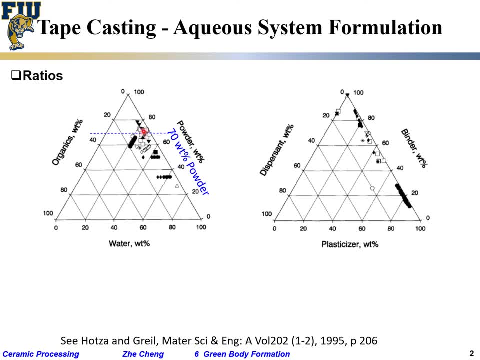 No, you cannot, You have to. you have to cut it in a different way Here, when I do powder, you see, my cut is parallel to the. this base, Okay, This base- or I'm getting away from 100%, remember this point- is 100% powder, which. 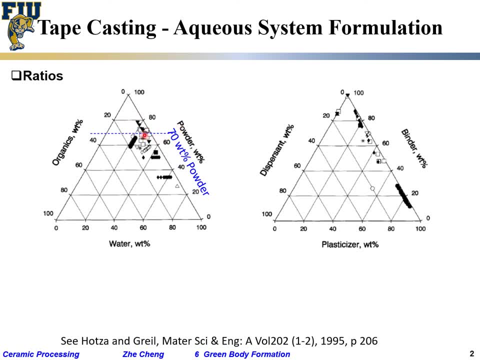 means this is 30% powder. Okay, And let's see to get organics. to get organics, I have to read this way and I have to do the cut: parallel to the base. Okay, Opposite to from, from this one: 100% organic. parallel to this guy, which means I have what? 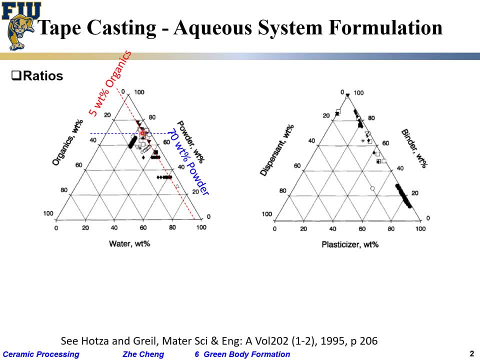 Five roughly 5% organics. instead of you read from here, You see what I mean When you cut this way: it's 70% powder but it's not 30% organic. You have to cut the other way to read what. 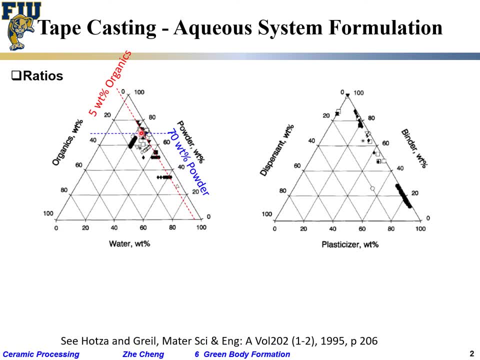 Organics. Pay attention, You cannot just go down: Okay, 30% powder, 30% organic. no, You have to cut the other way. Cut like this right away to read organics: Now it gives you 5% organics, because here is zero organics. 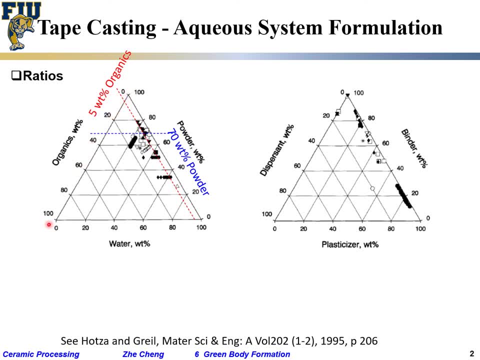 You see what I mean: Zero organics, and then you go to here, I become 100 organics. Of course, if I cut it from here, this is only 5% organic Make sense. And then, of course, to get the water. to get the water, can I read from here: 95% water. 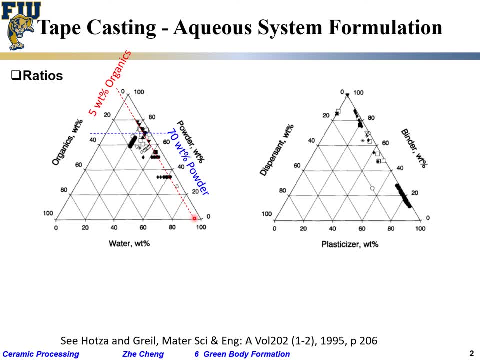 No, because I'm already what 75,, 70% powder. I cannot have 95% of water make sense. So to get the water content you have to cut still another way, parallel to that axis, getting away from 100% water. 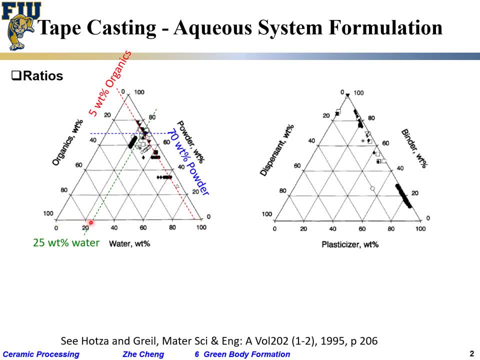 Now you read: 0% of water, 20% of water, 25% of water. You see what I mean. You see what I mean. So kind of like, be very, very careful, okay here. 70% of powder. no, it doesn't mean the. 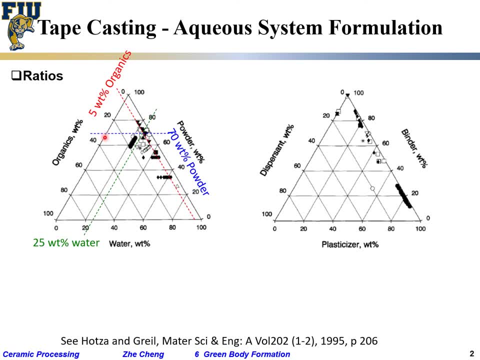 rest of 30% is all organics. you cannot read To organic. you have to cut in a different way To get water. you have to still cut another different way. Make sense: Now you get water, is 25% water? make sense. 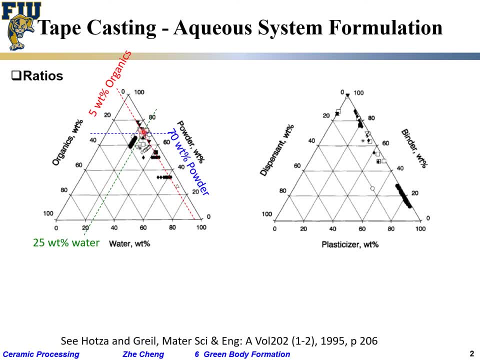 So this is kind of the thing. okay, this is my recipe. what is my recipe? I have roughly, I have in this case 78% of powder by weight, 5% of organics. the rest 25% is water. make sense. 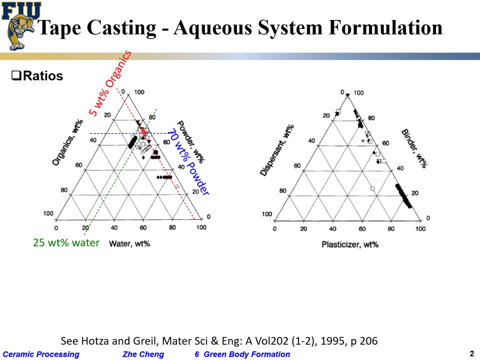 That's kind of one recipe, representative recipe. okay, So if I'm here, If I'm here right, If I'm here, from organics point of view, how much of organics? I mean, if you're right there, it's going to be 60% organic, 40% water and 20% water. 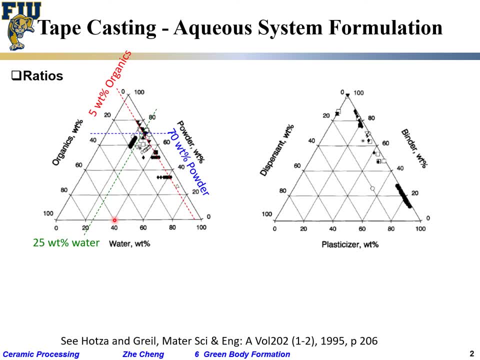 yeah, Right, Yeah, Even if I'm here, Yeah, Yeah, In terms of powder. in terms of powder, I have you remember: this is 100% powder. This side is zero powder. If I'm here, I have how much powder. 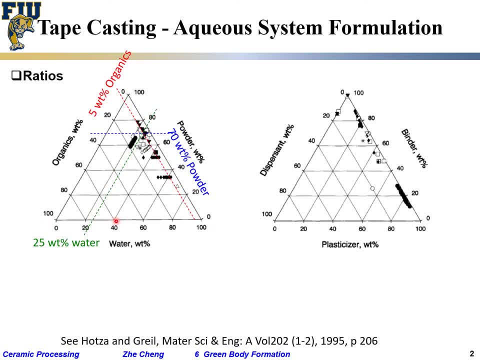 Zero, Zero powder. Make sense. I have zero powder Because this side is my 100% powder. if I'm here, I have zero powder, And then I have 40 and 60, right? So if I'm reading water, I'm 40%, right? 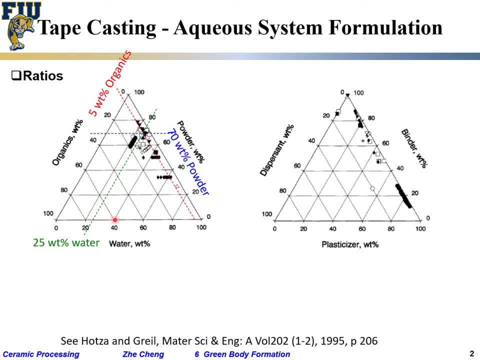 Yeah, Yeah, Yeah, Yeah. So I have 40% of water. Remember where is water? The water is here is 100% water. So I'm 40% of water and the rest 60 would be. 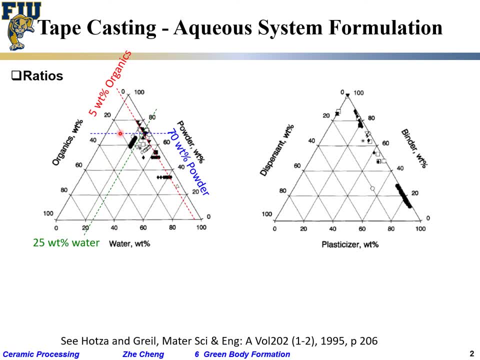 Organics, Organics, But in this case, because I'm so far away from remember, here is your pure powder and, as far as I can be away in this scale from Powder Powder, So I have zero powder Here. it's just I'm having a water-polymer mixture with, if you read, 40% of water make. 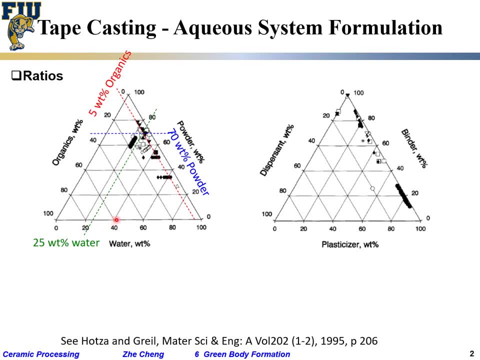 sense 40% of water and then 60% of organics. okay, So you can. in the same way, you can read the other plot, which is between all the organics. quite often you have dispersant, you have binder, you have plasticide, plasticide. 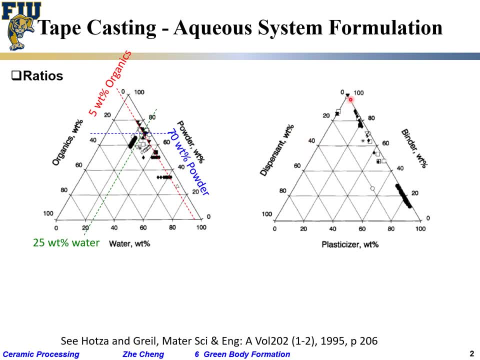 Dispersant. let's look at dispersant. if I'm reading dispersant from 0 to 100, so here means it's outward dispersant. but look at the actual formulation, The actual formulation in terms of dispersant. in most cases, the points are pretty far away.